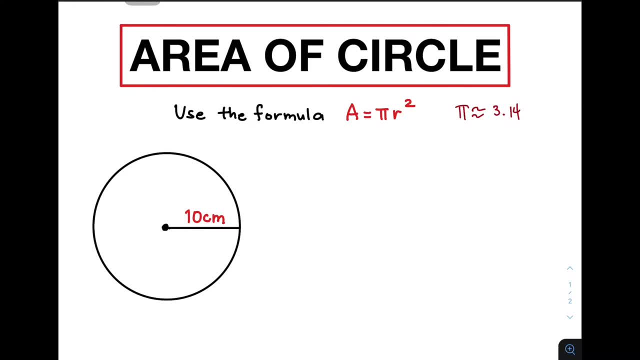 The first one is the Diameter. Diameter is a segment in which it connects two points, from one part of a circle to the other part of a circle, and it goes through the center. And the other segment that you need to remember is what you call the radius. 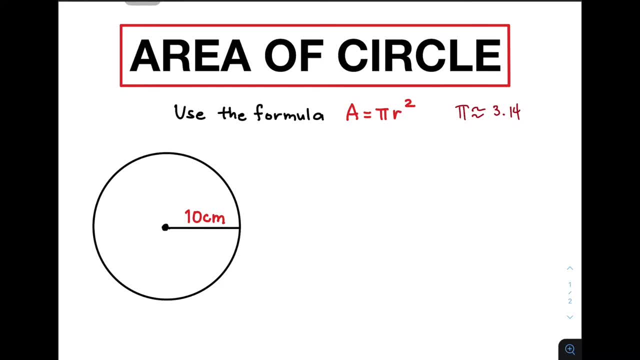 Our radius is a segment from one point of a circle up to the center, like this one. Okay, So know the difference. If this is the segment, this is your radius. And if you have a segment here from one point of a circle going to the second point of a circle and passes through the center, this is your diameter. 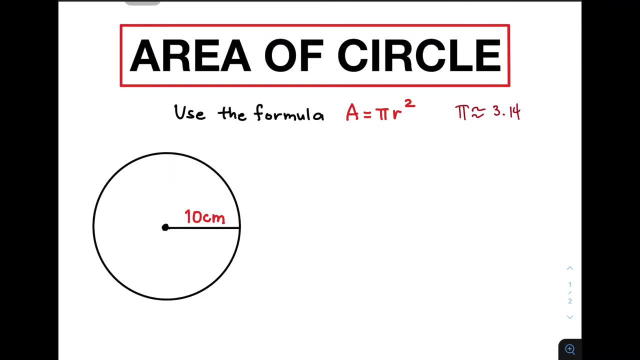 So let's start solving the area of the first figure. So we have here, in this given figure or in this given circle, we're in, We have the given radius, We have the given radius be equal to 10 centimeters. Remember, this is a radius. 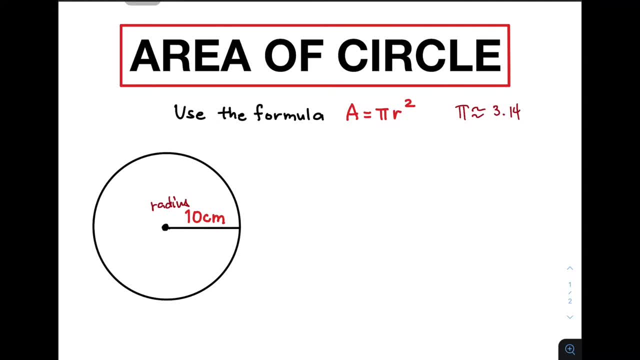 You have the radius, meaning your r is equal to 10 centimeters. So how are we going to calculate for the area of this given circle? Use the formula: area is equal to pi r squared. So first thing we need to do, some of the teachers. 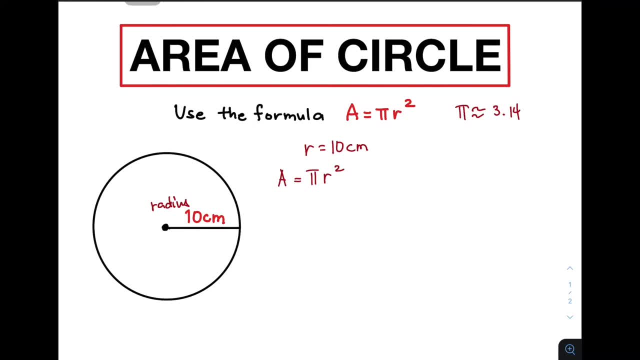 Are asking for the area of the circle, that we don't need to simplify the pi, And what we just need to do here is to simply plug in the value of r. So what we have here is that we have a is equal to pi times 10 centimeters squared. 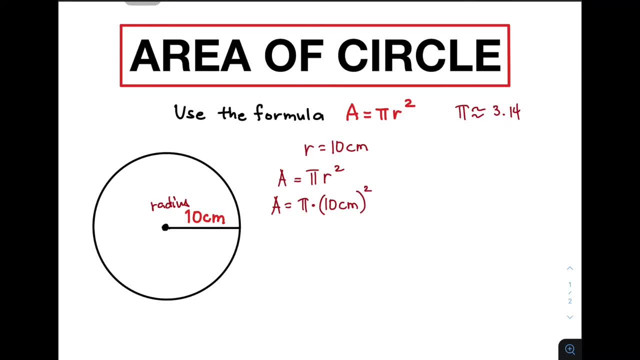 And simplifying this, your 10 centimeters squared is simply equal to 100 centimeters, Or 100 pi centimeters squared. So this is the area. Now, if your teacher wants you to simplify this one using this value of pi 3.14, we can still do it. 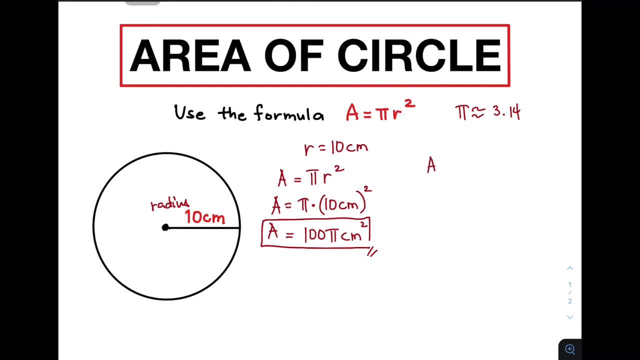 Simply by doing this, as area is equal to 100 times 3.14.. So this will give us the answer of: area is approximately 314 centimeters squared. As you can see, I have replaced this pi using the approximate value of 3.14.. 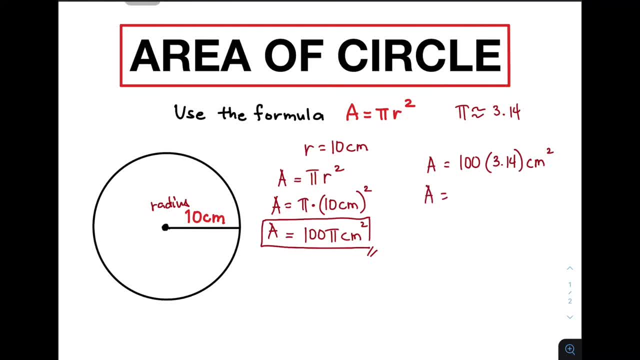 And this will give us the answer of: area is approximately 314 centimeters squared. So these are the possible answers in the first problem. So again, we use the symbol of approximately Approximation symbol, because the value of pi, which is 3.14, is an approximate value. 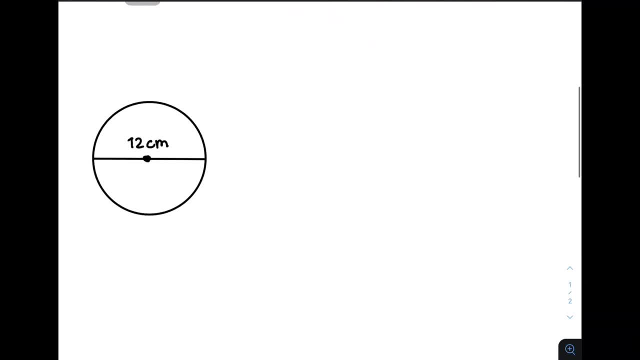 Now let's continue with our next problem. For the next problem, we are given this circle And, as you can see, this one is a diameter. So, in our formula we are using, area is equal to pi r squared. So, sir, how are we going to solve this? 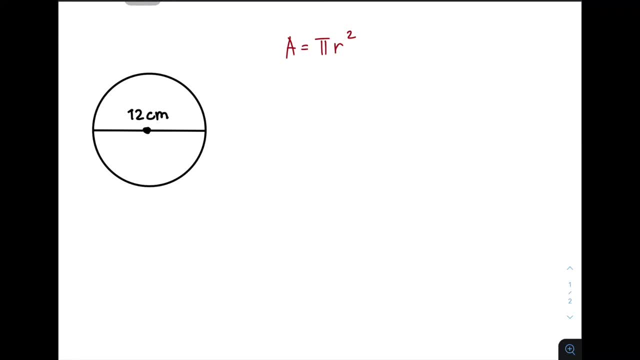 How are we going to solve for the area of this given circle if we have the diameter? Always remember that the value of your diameter is twice of the value of your radius Meaning. if you need the value of r, all you need to do is to use this formula. 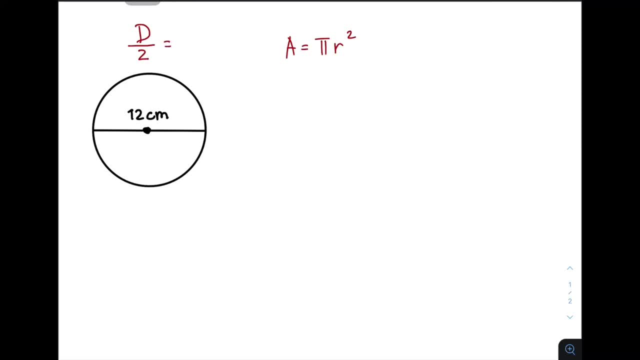 Your diameter is to be divided by 2, and that is equal to your radius. Again, let me write this one Again: your diameter divided by 2 is equal to the radius. So meaning, if your diameter is 12 and to simply get the value of your radius, 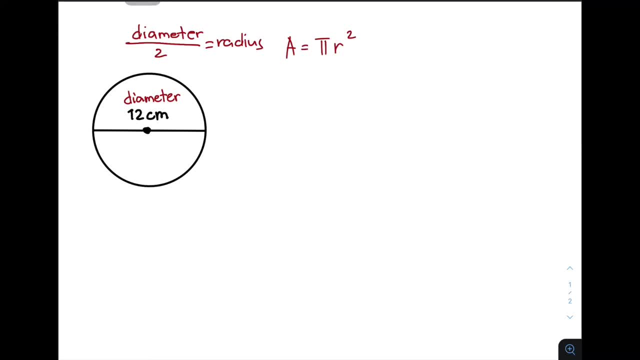 all you need to do is to divide this by 2 and this will give you the radius, or r is equal to 6 centimeters. So, using this formula, we need to plug in the value of r. We have a, or area is equal to pi times 6 centimeters squared. 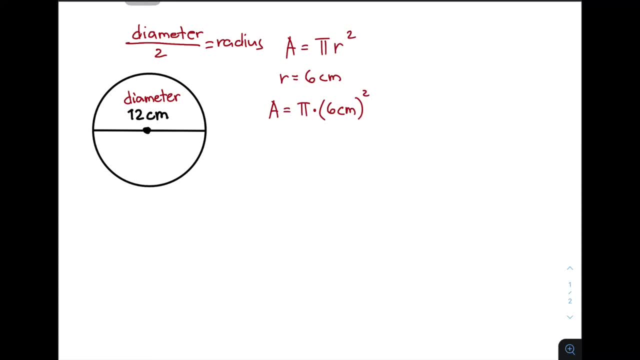 And we know that when we simplify this, this will give us 36 centimeters squared, And that will be area is equal to 36 pi centimeters squared. This is the first possible answer And if you will be using the value of pi, which is approximately 3.14,.